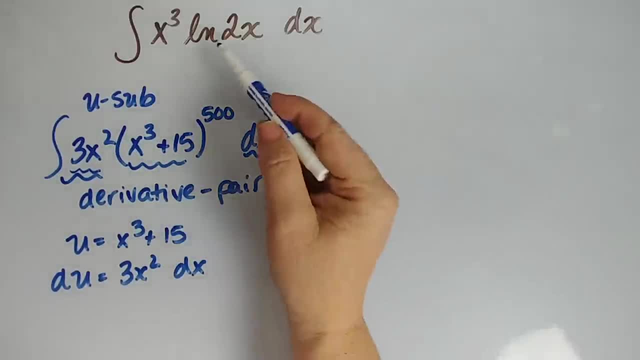 So u-substitution is going to be used there. So this: I see natural log of 2x. I know natural log derivative 1 over x. this is x cubed. I don't see a derivative pair, So u-substitution is just not going to work here. Okay, so then I go to my. if u-sub doesn't work because 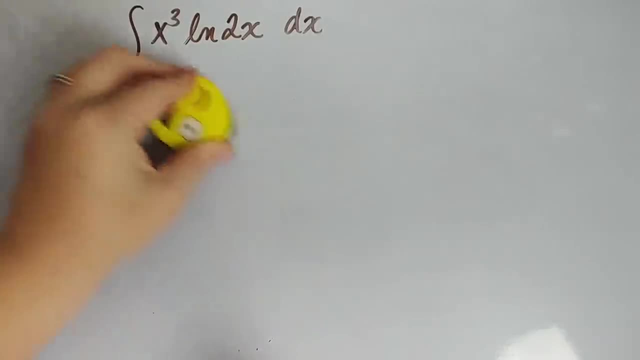 u-sub is generally the first one we learn, maybe the first one you check. It is a little easier, so I tend to check that first. It's easier to look for a derivative or a portion and a derivative pair. Okay, so then I'm going to go to, I'm going to go to, I'm going to. 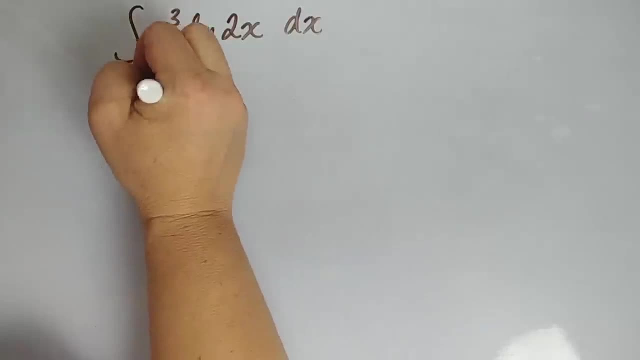 go to my integration by parts. My integration by parts says uv minus the integral of vdu. Okay, and that might not mean a lot to you. Basically, what we're going to do is we're going to call one part of our integral u and we're going to call the other part dv. 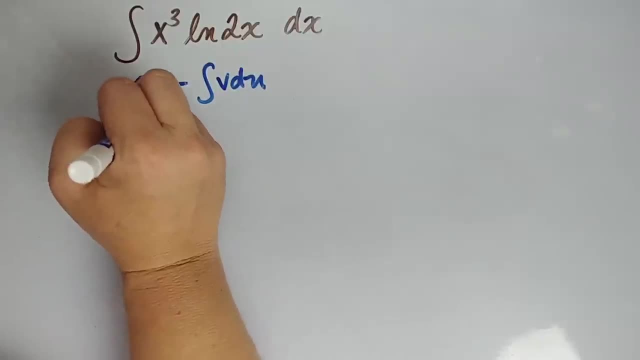 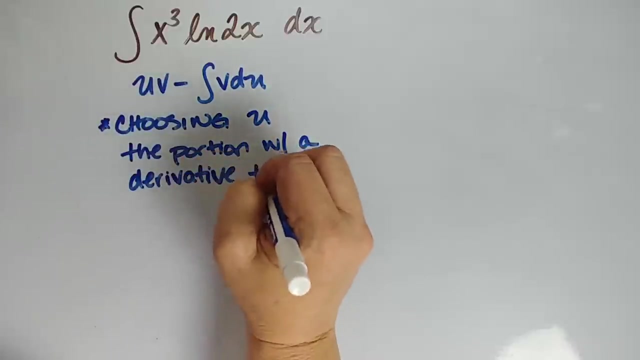 Now how to choose. So this is important: Choosing which part to call u You want. to choose the thing, you want, the portion that if you were to instead deal with its derivative, So the portion with a derivative that is nicer to deal with And that's nicer we'll put in. 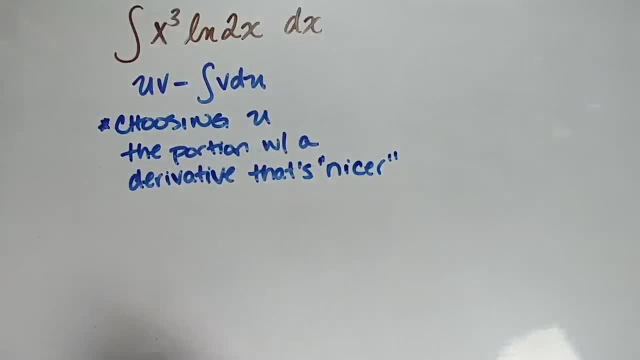 quotes: Okay, so something that's nicer to deal with. So, for example, looking at this, we have x cubed and we have the natural log of 2x. Well, if we let u be x cubed, then du is going to be 3x squared dx. 3x squared's not ugly. 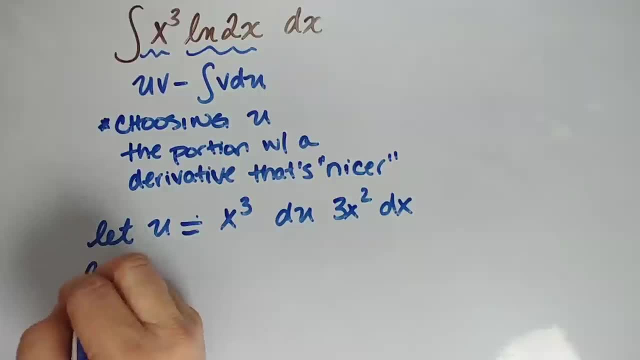 But it's not any nicer than x cubed. So let's see what happens if we let u instead be the natural log of 2x. Well then, du remember, it's going to be a chain rule here. We're going to say 1 over 2x times the derivative of the inside. So what, we're taking the. 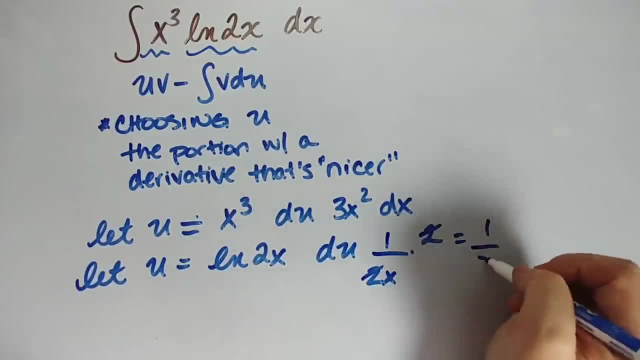 natural log of which is 2, so we just get 1 over X DX. I don't know about you, but 1 over X? DX is way nicer and easier to deal with then the natural log of 2x. and why do we want it to be nicer? look, do is the thing we're taking, the integral of. 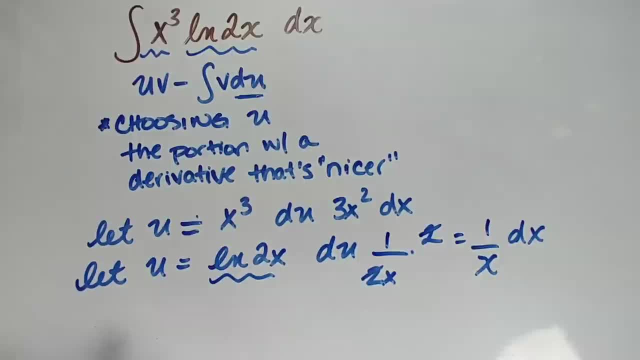 right, we got V, do? we're taking the integral of? so we want it to be nicer, easier to deal with, so we're definitely going to let you be this natural log of 2x and that's generally what I look at. I'm going to look at the two portions. 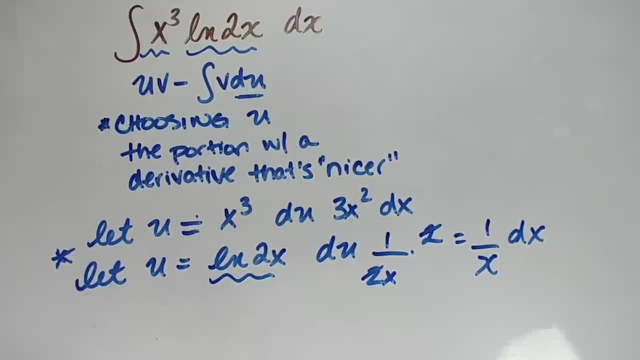 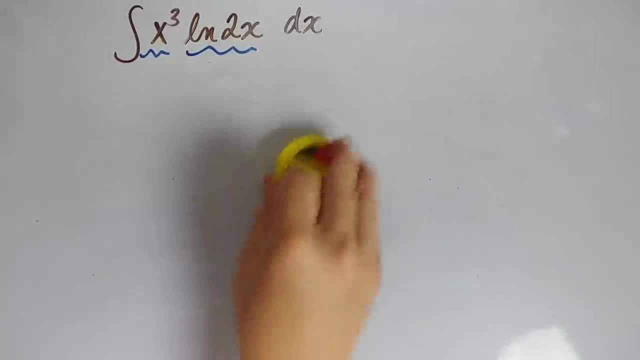 of my integral and say, hey, which of these is nicer if I were dealing with its derivative rather than it? all right, so let's get rid of all of this now. well, probably could have kept the formula there, that's okay, we'll write it again. okay, integral integration by parts is UV minus the integral of V. do we already? 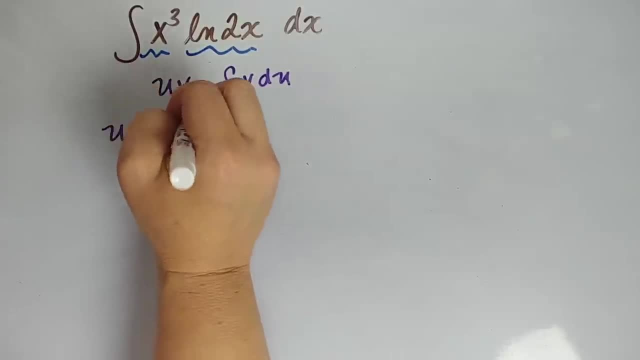 said, we're going to let you be the natural log of 2x, because then do is 1 over X, DX. okay, my DX is a little messed up there, all right. and so then, um, we're gonna say, well, what are we gonna let B DV, well, DV, and a lot of people put DV here because 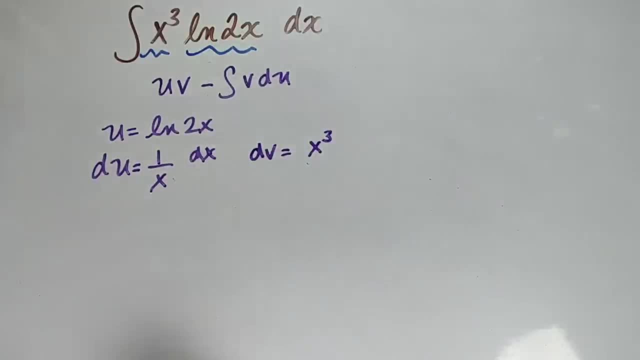 what happens is if we let X cubed B, DV, we are actually going to integrate to get back to V. so, derivative of V, you integrate to get back to V and that is basic integration rule. you're going to take your power, increase the power and divide it by that new power. so V is going to be X to the fourth over four. 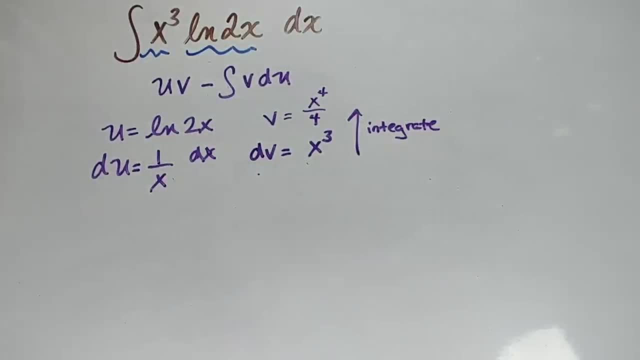 okay, so far so good, all right. so now we really can just sort of plug it all in. so let's do that. so we've got UV. well, U is the natural log of 2x, so natural log of 2x times V, so times V, V. is this X to the fourth over four, or 1 fourth X to the? 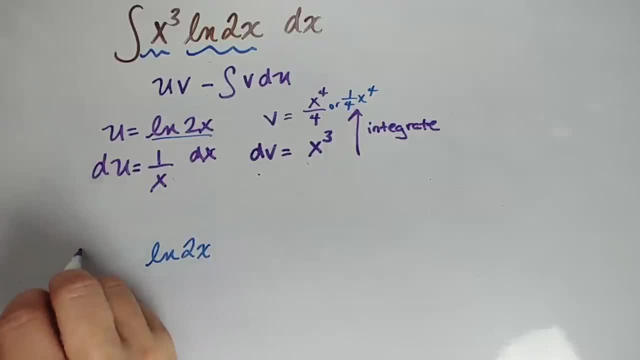 the fourth, And that's what I'm going to use And I'm actually going to put it right here: One fourth x to the fourth times the natural log of 2x minus the integral of v, du. So v again is one fourth. 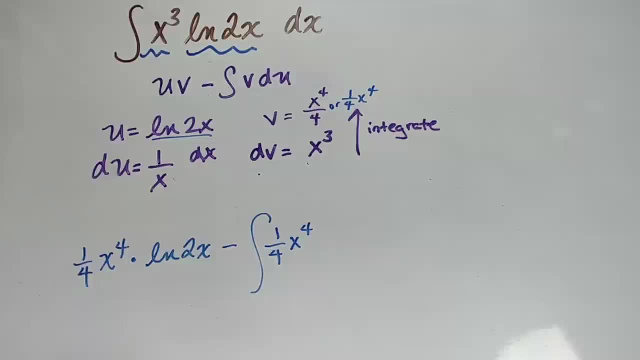 x to the fourth, du. Remember du is the thing that became easier. So one over x dx. All right, We are going to clean this up for sure. For right now I don't love it, So let's say I'm not going. 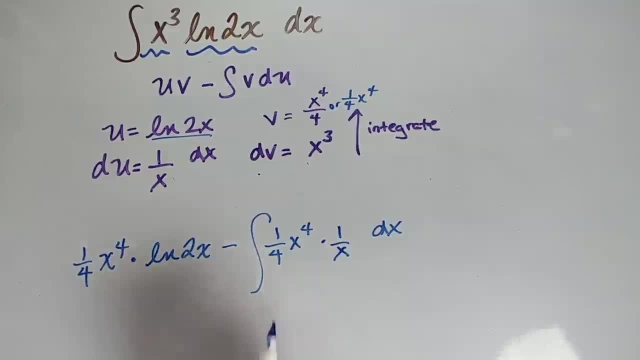 to do much to the left side. I'm going to kind of keep the left side as is. I'm going to pull out this one fourth here And I'm going to say we're going to work with this little thing right here. So if we kind of come over here to the side, we say the integral of one fourth. x to the fourth. 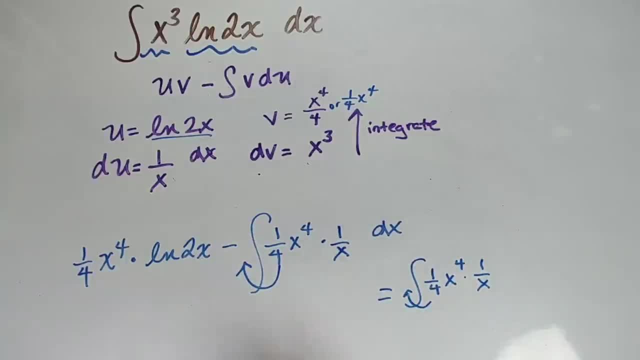 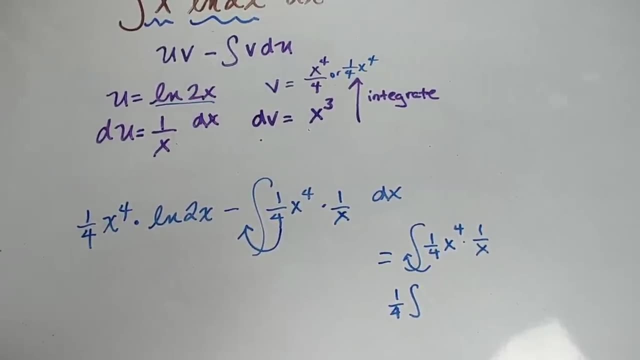 times one over x. We really pull out one fourth Right. So one fourth times the integral, Let's bring that back. So we're going to pull out one fourth times the integral, Let's bring that back. I'm going to bring this down a little bit before you can't see what I'm doing. And then x to the. 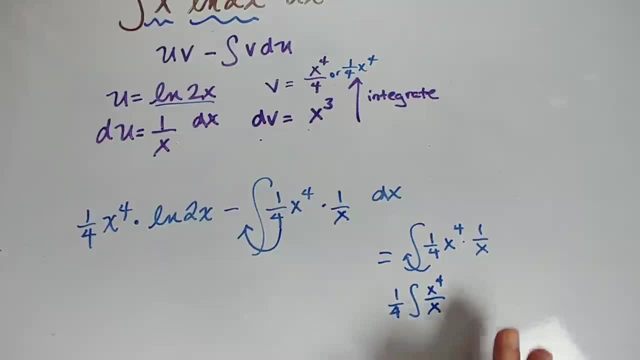 fourth times. one over x is x to the fourth over x, which we all know is x cubed. Okay, So this thing is x cubed, All right, So that's what I'm going to turn this thing into. So let's bring out my one. 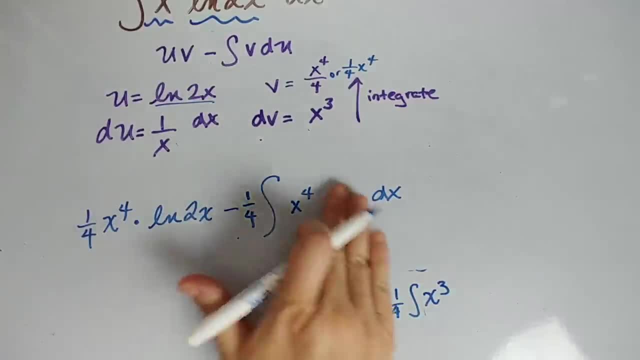 fourth, My integral sign goes back. This becomes x cubed dx- The beauty of a whiteboard. Okay, Now I can do something with this. All right, So we're going to nothing's happening over here. Normally I'd say, okay, do x to the fourth times. natural log of x all over four. But I'm not going. 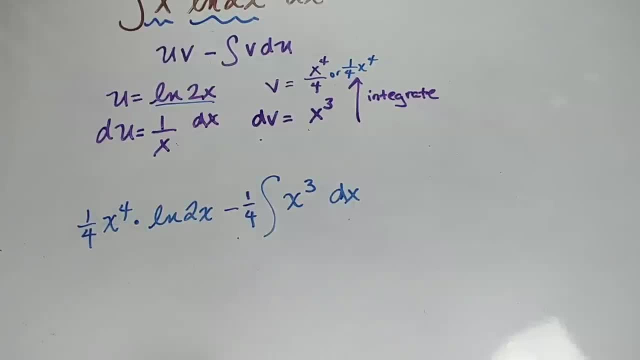 to, And I think you're going to see why actually very shortly. So let's just make it. you know, clean it up a little bit. We're just going to get rid of our dot for multiplication Minus one fourth. Okay, So minus one fourth, And then we have that x cubed. Well, we already know to take the integral. 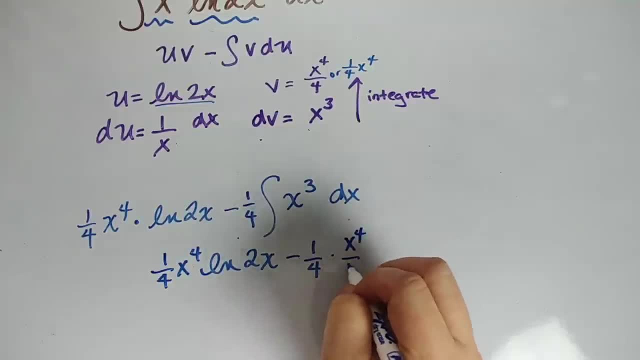 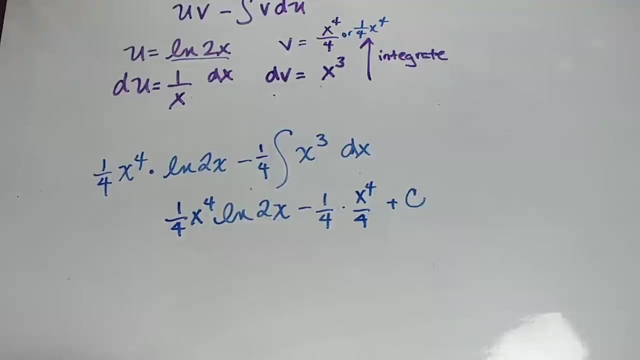 We say x to the fourth, all over four plus c. Okay, So now you're thinking we're done- Yeah, we're not done. Or you might be thinking we have to clean this up, We have to multiply this And normally you'd be on the right track. Okay, Multiplying those and getting one fourth. x to the fourth. 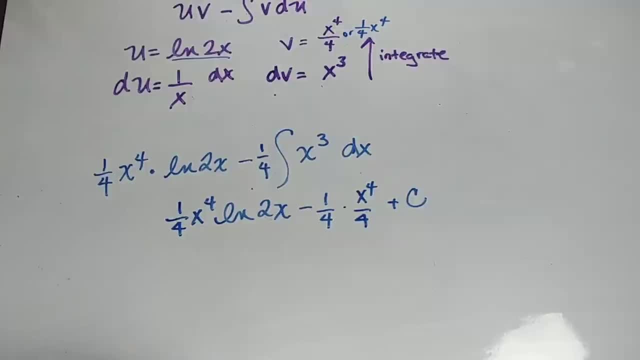 times natural log of 2x minus maybe x to the fourth over 16 plus c, But generally speaking, teachers and textbooks do one thing When they see something that's repeated. A factor, Remember one fourth. x to the fourth is the same as x to the fourth over four. 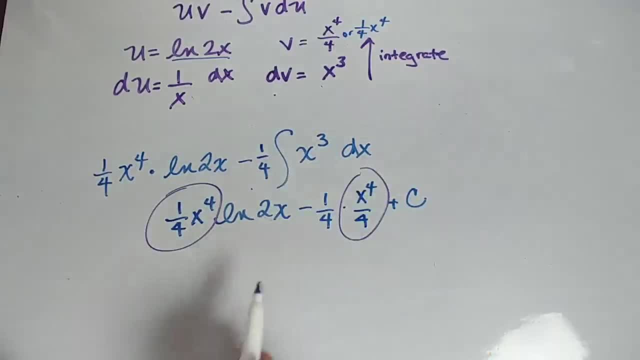 So the fact that I've got this factor in both of my terms- Remember, here's my subtraction sign, So I have two terms here- Means I can take this factor out. So I'm going to do that. So I'm going to take. 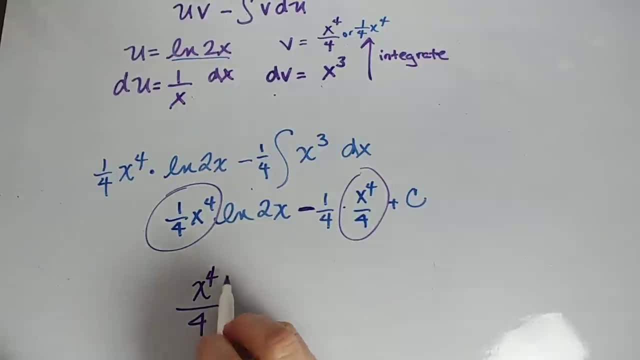 x to the fourth over four out. And what am I left with? I'm left with natural log of 2x minus one fourth plus c. Okay, And my plus c, really, I could have just waited to the end to put it in, in case you said: 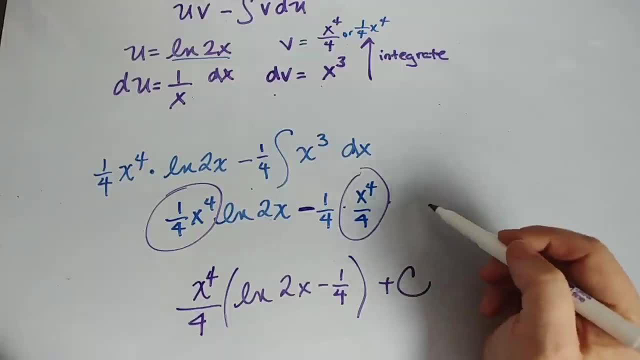 hey, listen, you took something from a factor that wasn't in the c. Remember, a c is just your constant plus any constant doesn't change the answer to this. So we really could have just left the adding the plus c to the end. So this is okay if I just kind of put a plus c here and 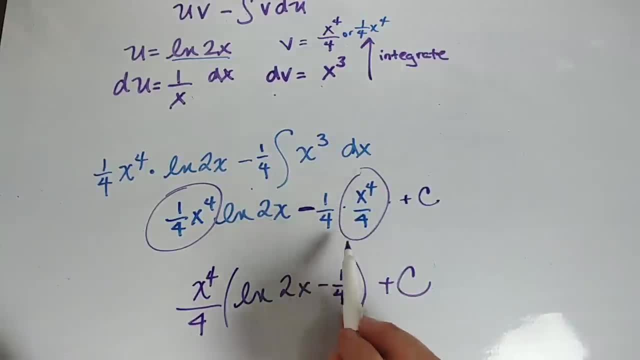 left it final. Maybe I would have multiplied this x to the fourth over 16.. I really don't think that's what your textbook answer would look like, though, because teachers and textbooks are kind of, because it's nice and neat and puts everything in a cute little package. so 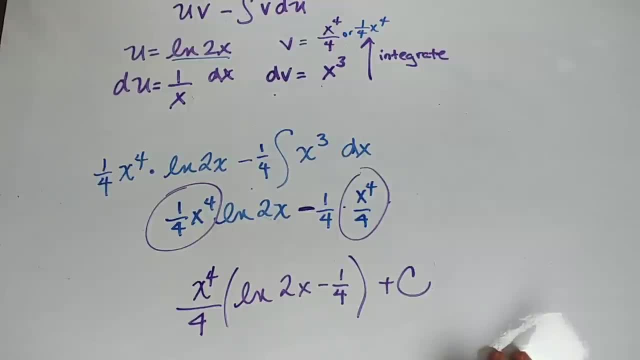 you're done here. you know when to use you substitution. you look at it, something, and you see its derivative sitting there. use you substitution generally if you can't use that. parts is a good idea. you wanted to say, hey, what's going to be you, what's going to be DV? you is the thing. that would be way easier if they had. 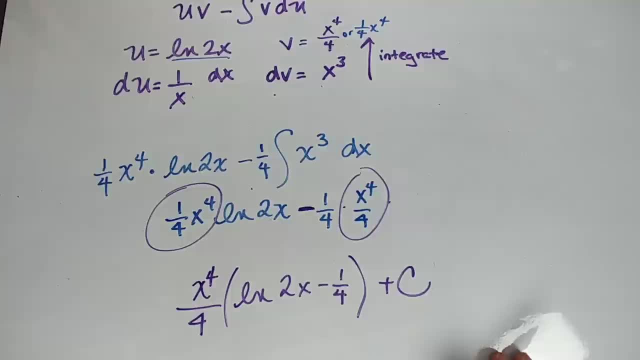 given you the derivative because that's what you're going to use. I hope this helped place your comments or questions in the comment section. be sure to like the video, be sure to subscribe to our YouTube channel and go ahead and send us your problem next time you get stuck.